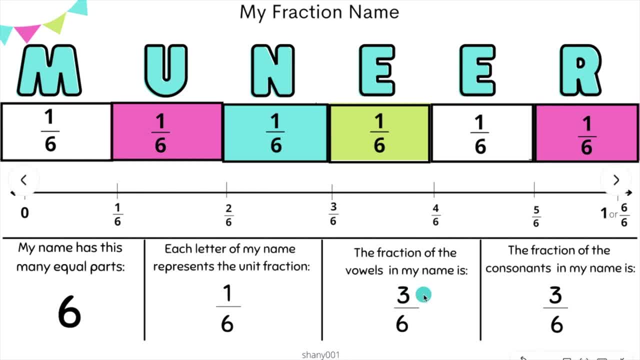 in my name. My name has three vowels. Vowels are the letters A-E-I-O-U, So I have the letter U-E-E, So that makes my fraction three-sixth. The fraction of the consonants in my name is also three-sixth. Anything that's not a vowel, such as the letters N-N-R. 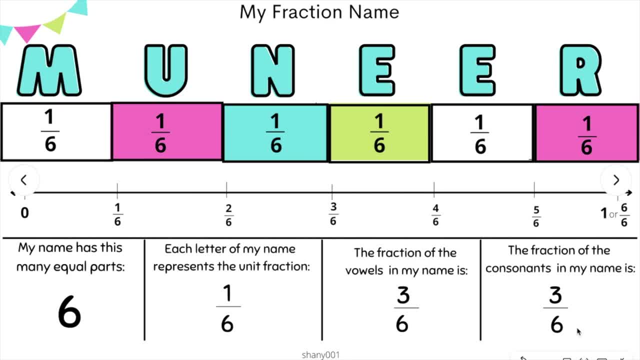 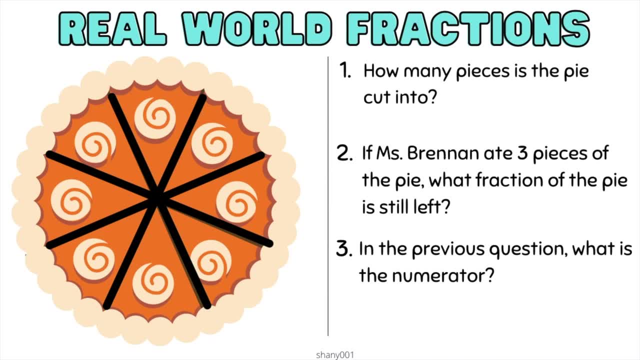 make my fraction three-sixth as well. In this example, we are cutting pie. Number one: how many pieces is the pie cut into? Number two: if Miss Brennan ate three pieces of the pie, what fraction would it be? And number three: how many pieces does the pie cut into? 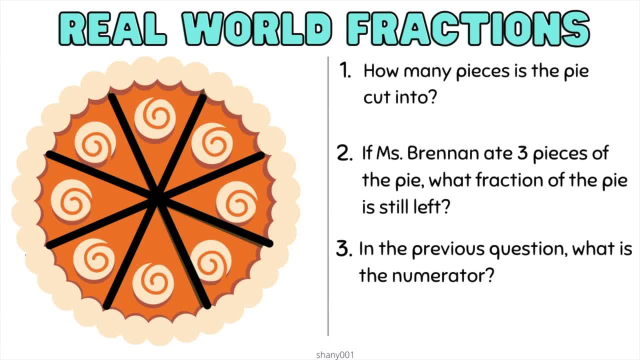 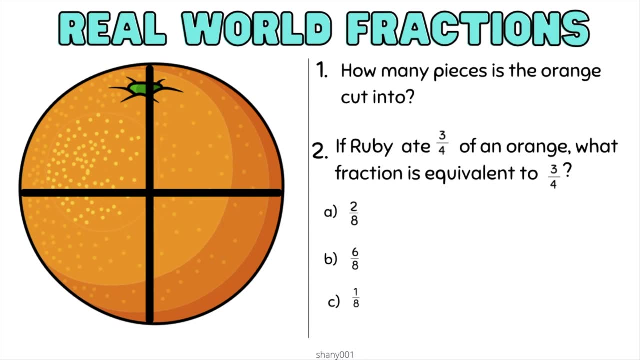 The fraction of the pie is still left. Number three in the previous question: what is the numerator? In this example, we are cutting an orange. Number one: how many pieces is the orange cut into? Number two if Ruby ate three? what fraction would it be? And number three: how many pieces does the pie cut into? The fraction of the pie is still left. Number three: how many pieces does the pie cut into? The fraction of the pie is still left. Number four: how many pieces does the pie cut into? The fraction of the pie is still left. Number five: how many pieces does the pie cut into? The fraction of the pie is still left. Number six: how many pieces does the pie cut into? The fraction of the pie is still left. Number seven: how many pieces does the pie cut into? The fraction of the pie is still left. Number eight: how many pieces does the pie cut into? The fraction of the pie is still left. Number nine: how many pieces does the pie cut into? The fraction of the pie is still left. Number ten: how many pieces does the pie cut into? 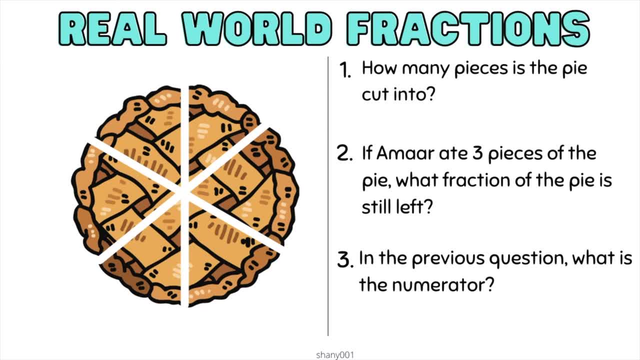 In this example we are cutting pie. Number one: how many pieces is the pie cut into? Number two: if Amar ate three pieces of the pie, what fraction of the pie is still left? Number three in the previous question. what is the numerator? 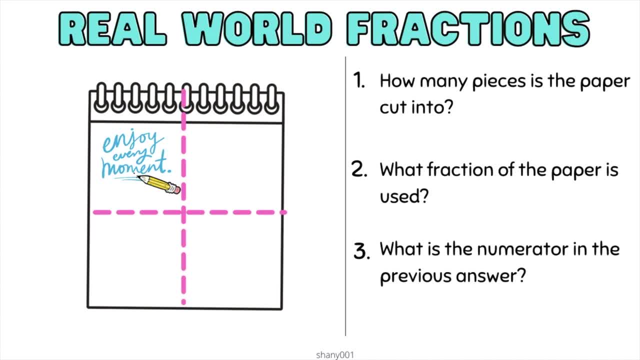 In this example, we are cutting a piece of paper. Number one: how many pieces is the paper cut into? Number two: what fraction of the paper is used? Number three: what is the numerator in the previous answer? In this example, we are cutting lasagna. 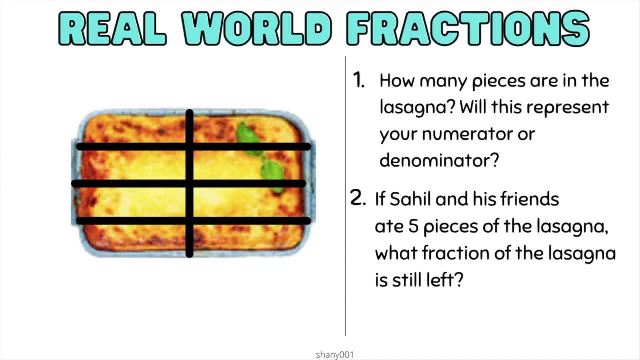 Number one. Number one: how many pieces are in the lasagna? Will this represent your numerator or denominator? Remember, when you're talking about all the pieces, the total pieces, it usually is your denominator. Number two, if Sahil and his friends ate five pieces of the lasagna, 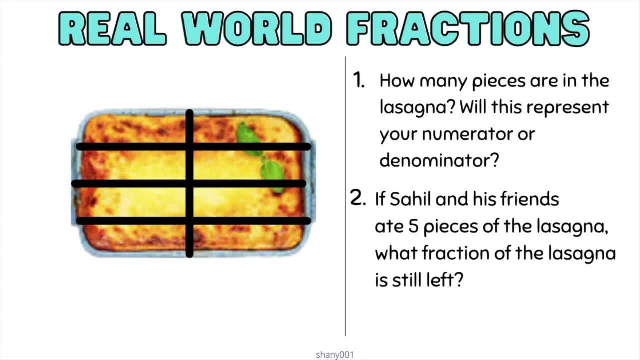 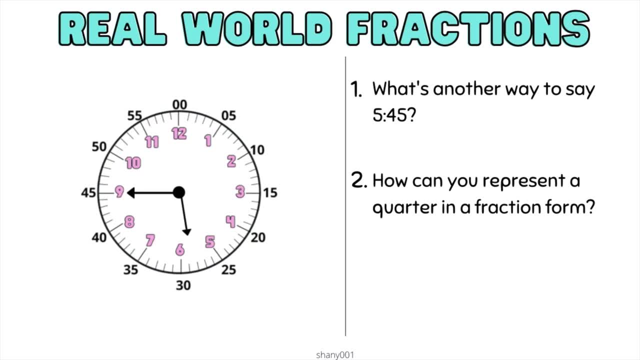 what fraction of the lasagna is still left? What fraction of the lasagna is still left In this example? we are telling time. Number one: what's another way to say 545?? Number two: how can you represent a quarter in a fraction form? 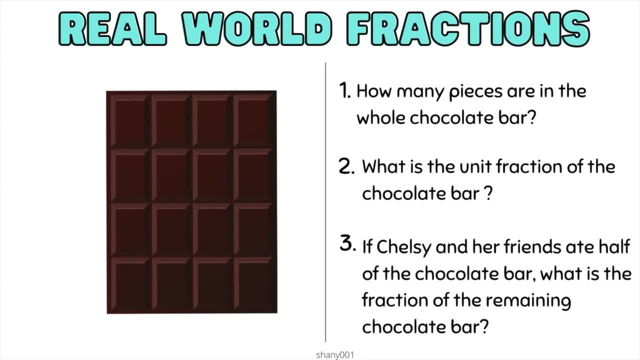 In this example we are using a chocolate bar Number three. how can you represent a quarter in a fraction form Number one? how many pieces are in the whole chocolate bar? Number two, what is the unit fraction of the chocolate bar? 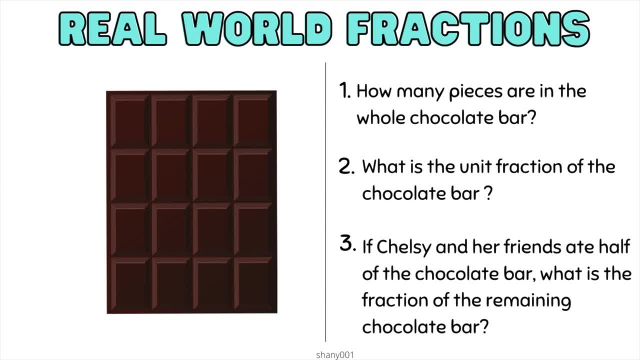 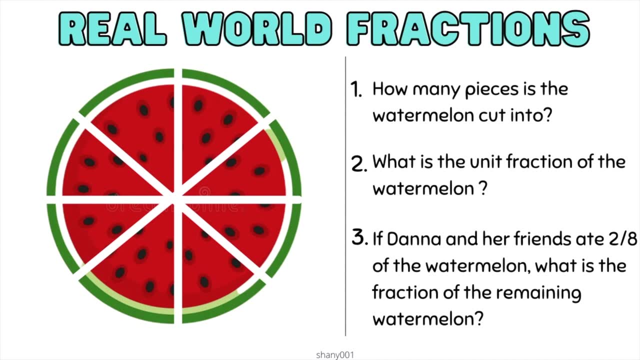 Number three: if Chelsea and her friends ate half of the chocolate bar, what is the fraction of the remaining chocolate bar? In this example, we are using a watermelon. How many pieces is the watermelon cut into? Number two: what is the unit fraction of the watermelon? 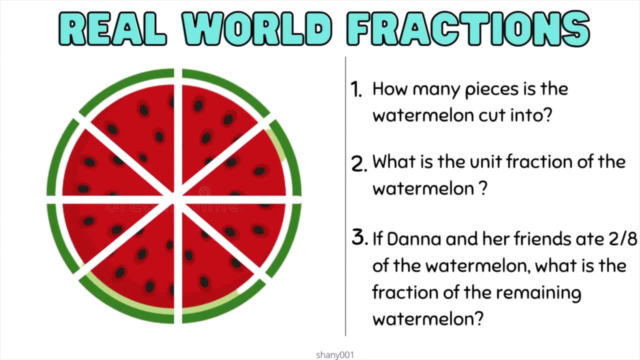 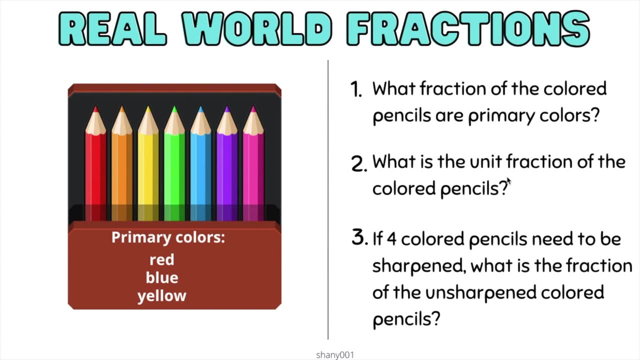 Number three: if Dana and her friends ate two-eighths of the watermelon, what is the fraction of the remaining watermelon? In this example, we are using colored pencils. Number one: what fraction of the colored pencils are prime? Number two: what is the unit fraction of the watermelon? 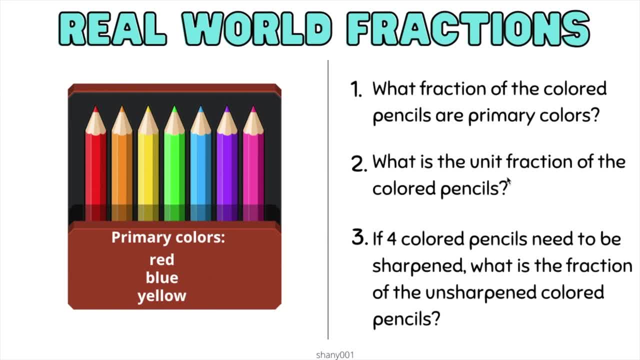 Remember, primary colors are red, blue, yellow. Number two: what is the unit fraction of the colored pencils? Number three: if four colored pencils need to be sharpened, what is the fraction of the unsharpened colored pencils? 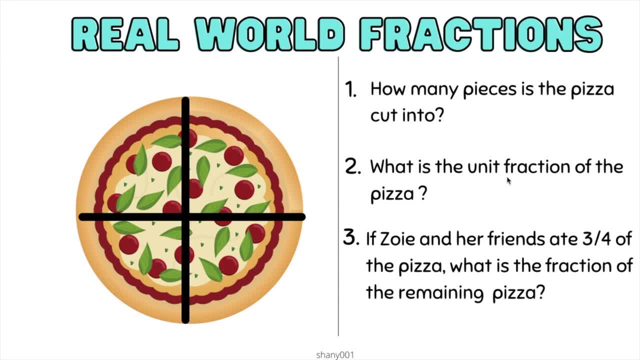 In this example, we are eating pizza. Number one: how many pieces is the pizza cut into? Number two: what is the unit fraction of the pizza? Number three: if Zoe and her friends ate three-fourths of the pizza, what is the fraction of the remaining pizza? 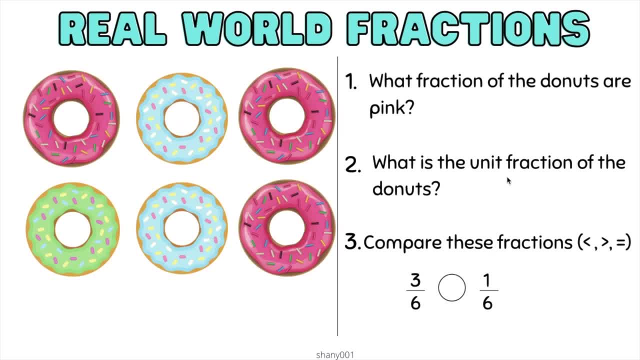 Number four: what is the unit fraction of the remaining pizza? In this example, we are eating pizza. In this example, we are using doughnuts. Number one: what fraction of the doughnuts are pink? Number two: what is the unit fraction of the doughnuts? 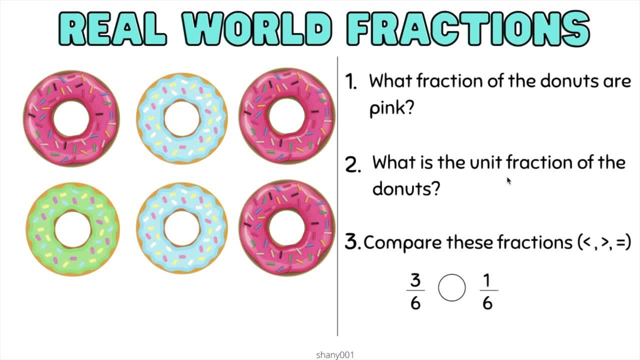 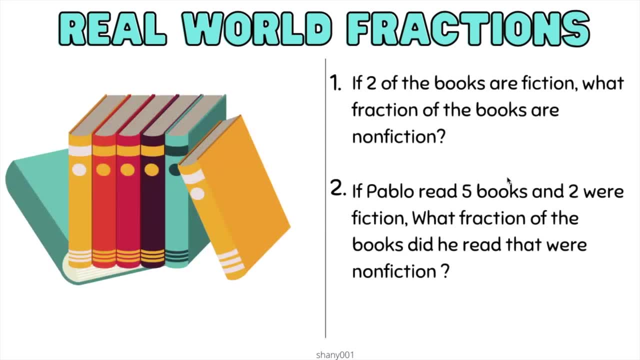 Number three: compare these fractions. In this example, we are using books. Number one: if two of the books are fiction, what fraction of the books are pink? Number two: what fraction of the books are nonfiction? Number three: if Pablo read five books and two were fiction, 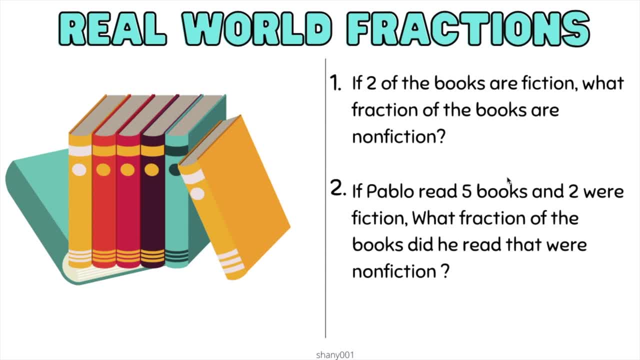 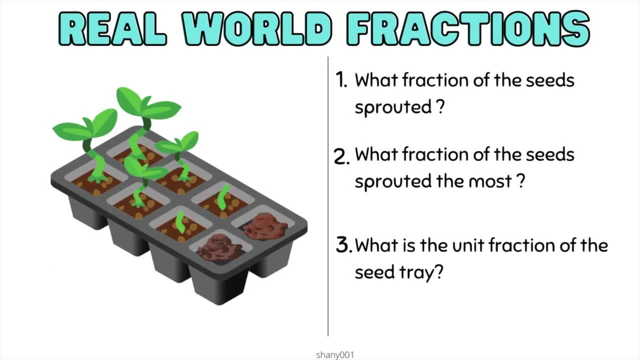 what fraction of the books did he read that were nonfiction? In this example, we are using a seed tray. Number one: what fraction of the seeds sprouted? Number two: what fraction of the seed sprouted the most? Number three: what is the unit fraction of the seed tray? 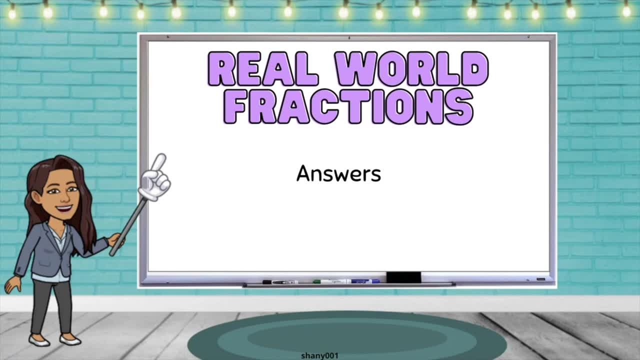 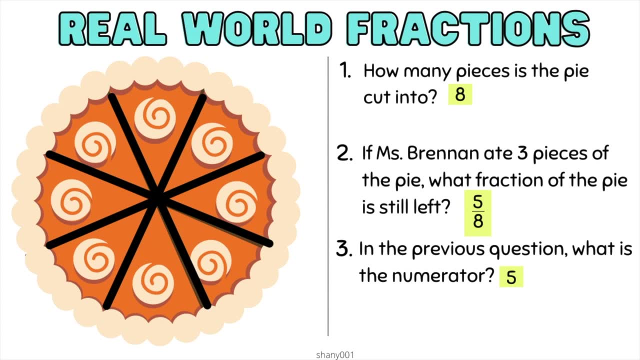 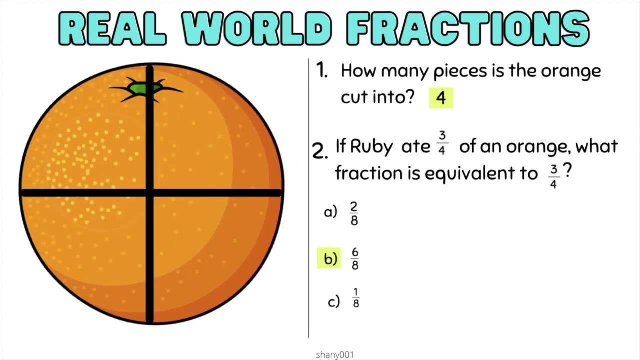 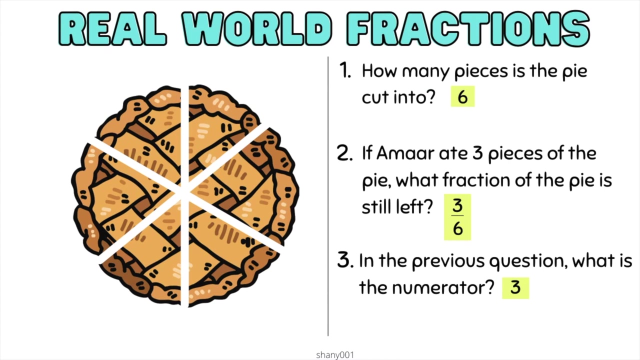 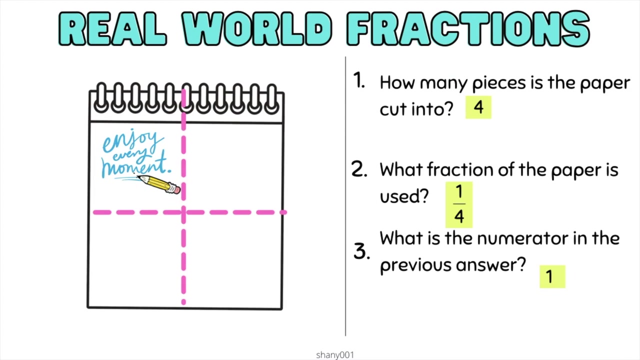 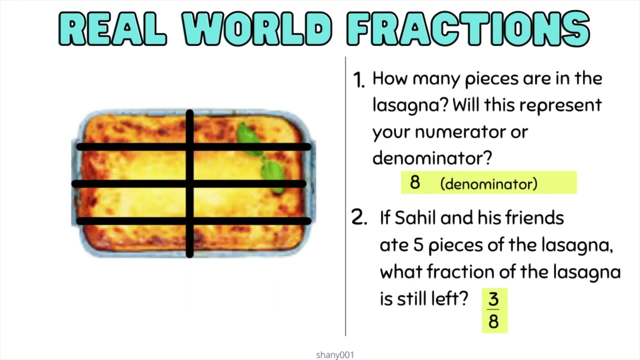 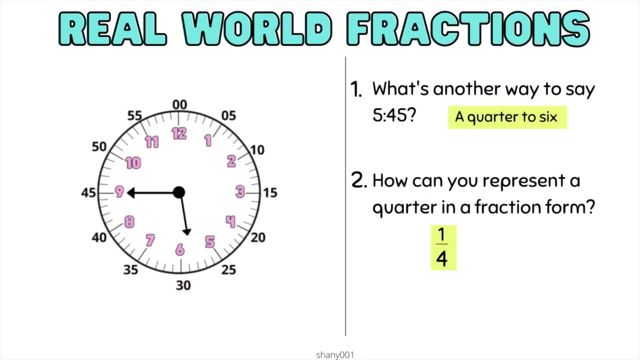 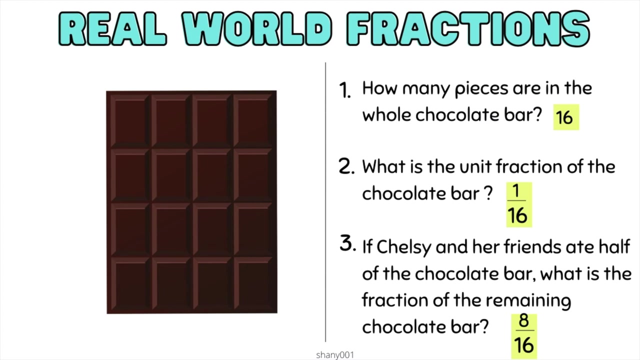 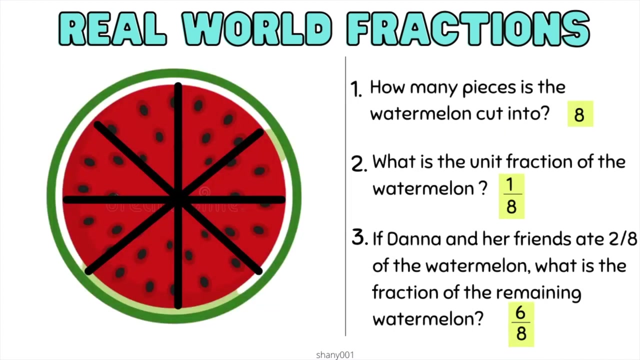 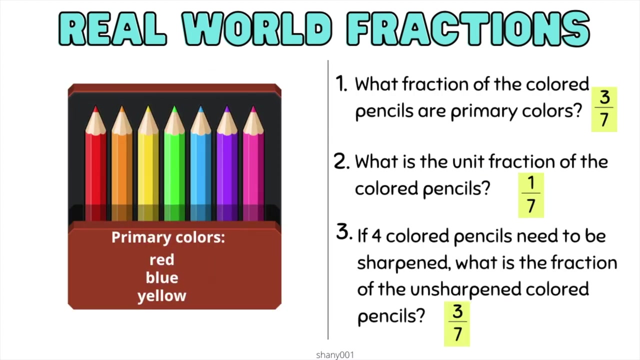 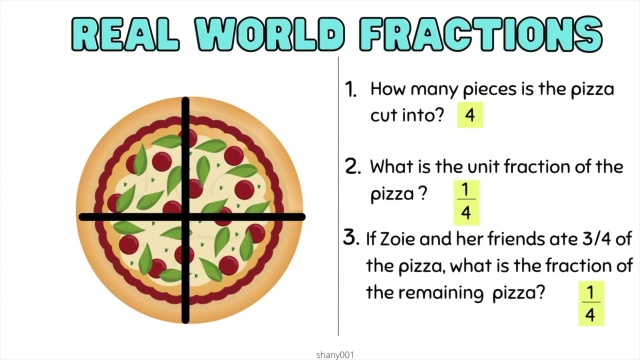 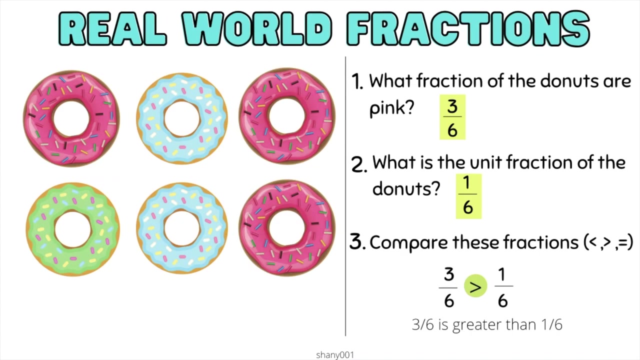 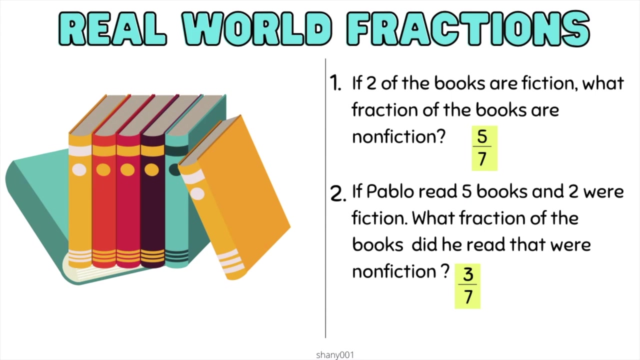 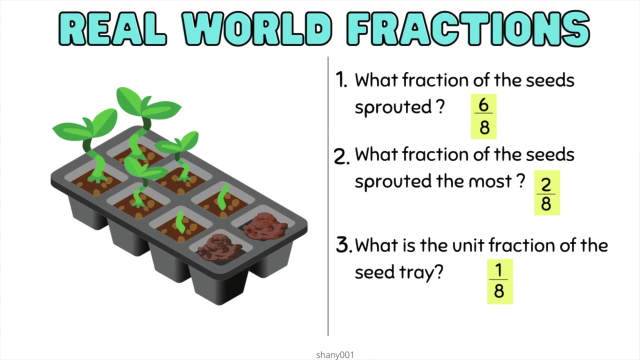 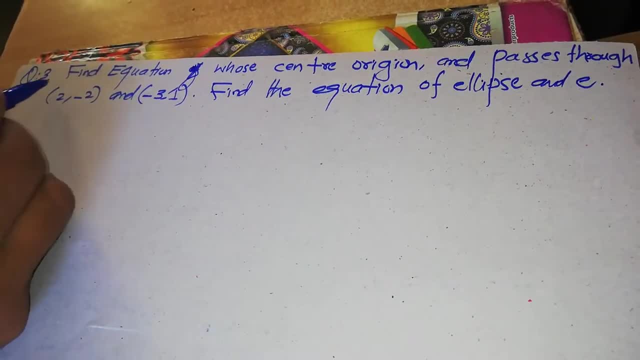 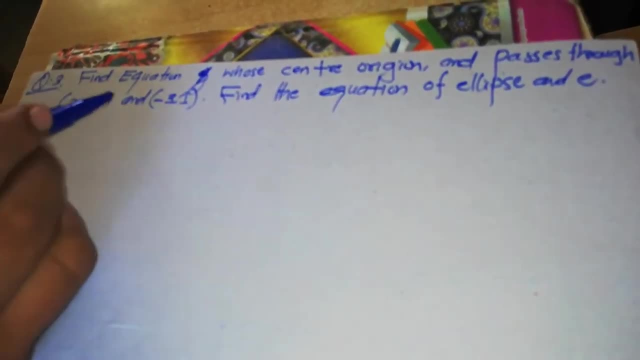 Now we will solve a question, number three of the conic section, which is find equation of the ellipse, whose center origin and passes through the points which are 2 minus 2 and minus 3 comma. 1. Find the equation of ellipse and E means. 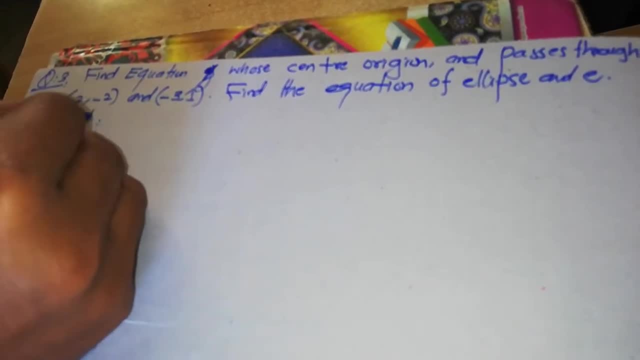 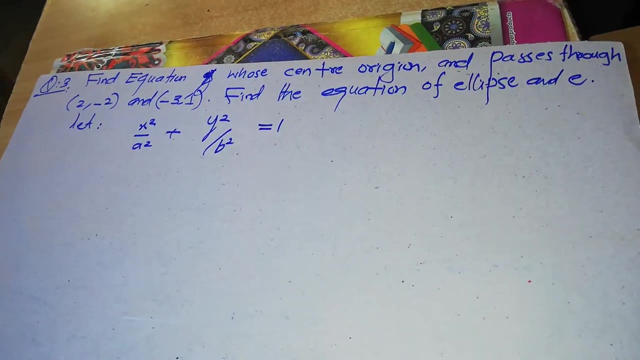 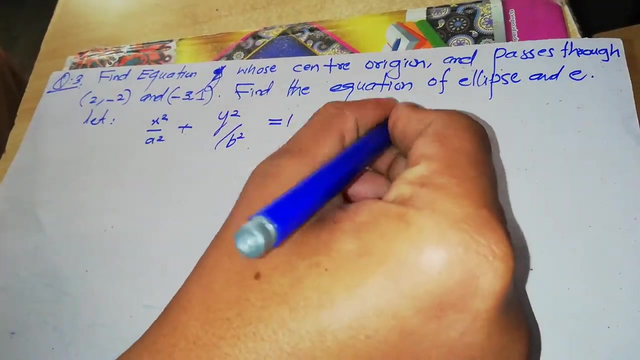 extensity Let. the equation is: x square over a square plus y square over b square is equal to 1. and here is a hint, which is that ellipse passes through 2 comma minus 2 and minus 3 comma 1, which means that we are taking the co-ordinates of point P. 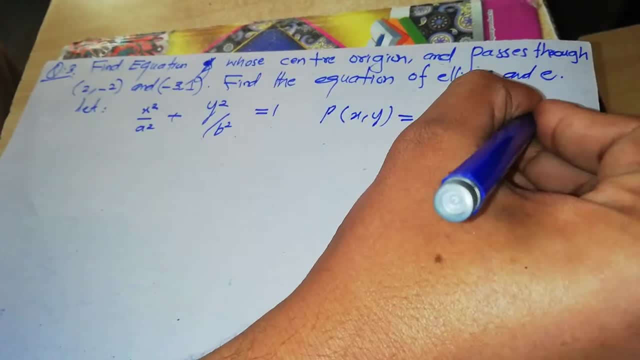 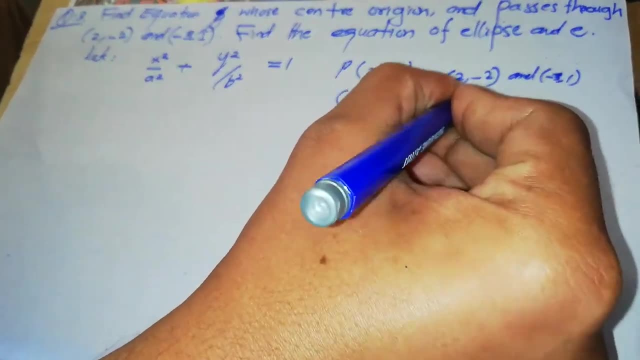 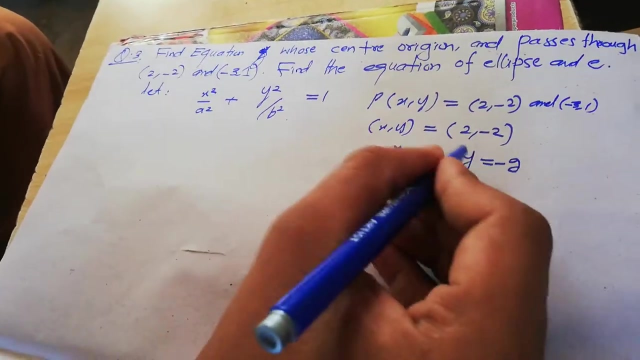 and first of all that we are using point P, that is, 2 comma 2, which means which equals 2 comma minus 2 k. Now the value of x is 2 and the value of y is minus 2. Put these points in general equations: What is value of X? 2 means 2 whole square.